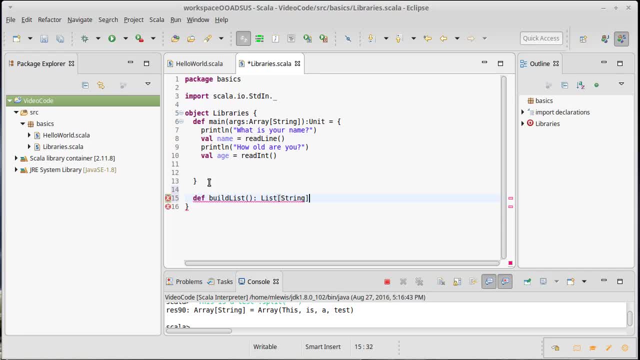 It's going to be a list. We will go with strings, And what I want to do here is I want to read from the user: So now, input equals readLine, And then I want to check If I'm saying quit, we're going to stop. 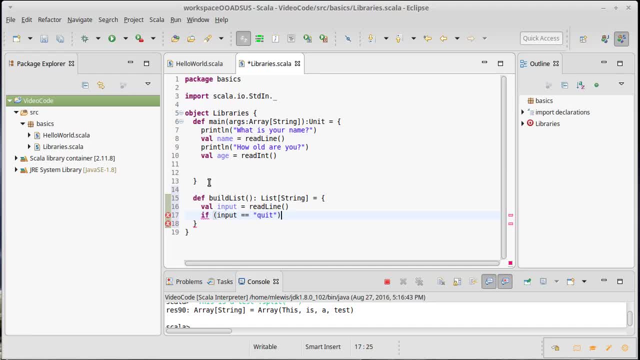 If input is quit, then I want to give them back an empty list. So you can imagine we've called this. They type in: quit, I'm going to give them back no list at all. Now I can say an empty list like that, but there's also a name for the empty list that we will use. 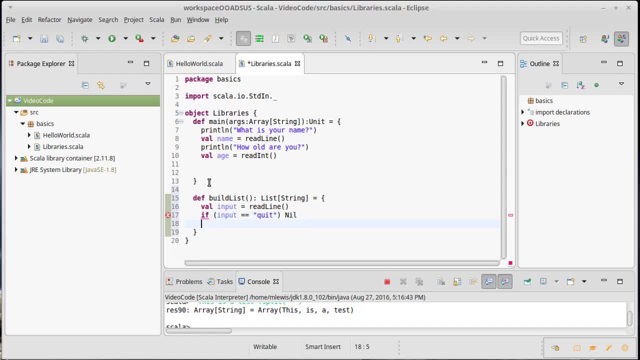 It's called nil- Notice it has a capital L there- And then we can say else. Well, what if the input isn't quit? Then I want to take that input and I want to give it back, consed onto the result of calling buildList again. 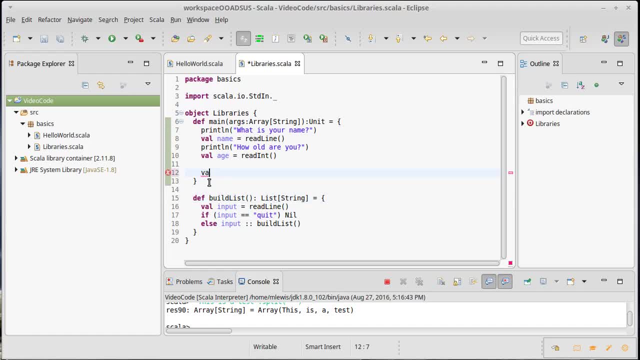 So we can show how this works. Let's go ahead and say: val lst equals buildList printLine lst. We can run that. Now it's still asking us, for example, for our name and our age. Okay, now it's asking us for just words, whatever. 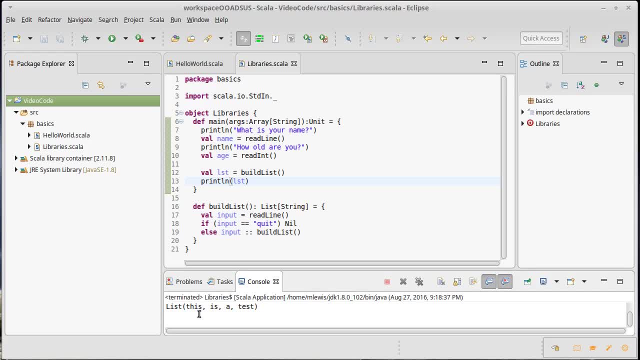 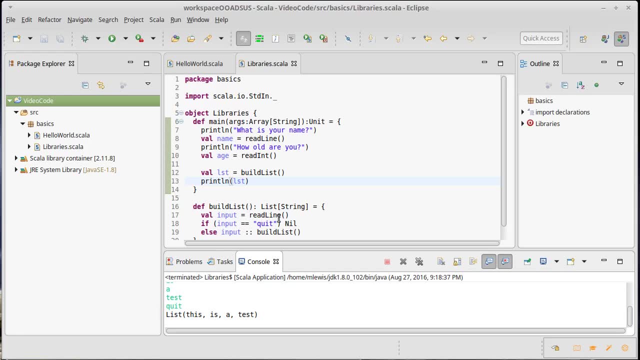 I didn't give it any prompts, so you can't really tell what it's asking. But I typed in this is a test And then I typed in quit, and so we get back that list. So here we're using cons in a recursive function. 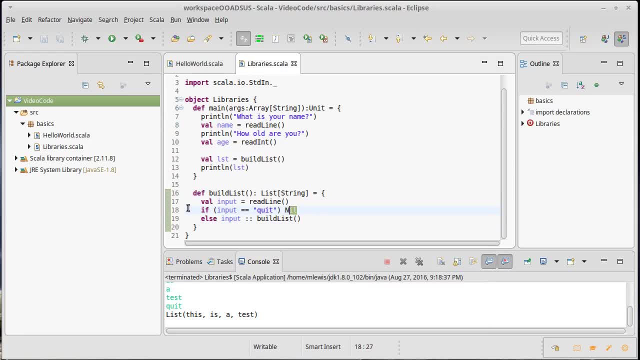 To build up a list. all recursive functions need a base case. So our base case here is nil. We've gotten to the end of the input and we just want to return an empty list And then at each time through it winds up adding an element to the beginning of the list that is kind of the rest of the list. 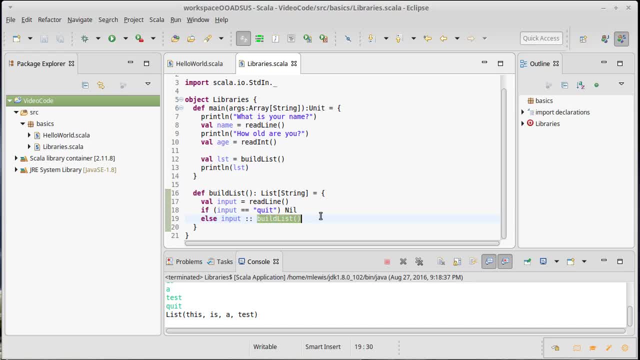 So you should think of it as this element consed onto the rest of the list And at the end the rest of the list is just an empty list. So that's an example of how you can use cons and a recursive function to put together a list. 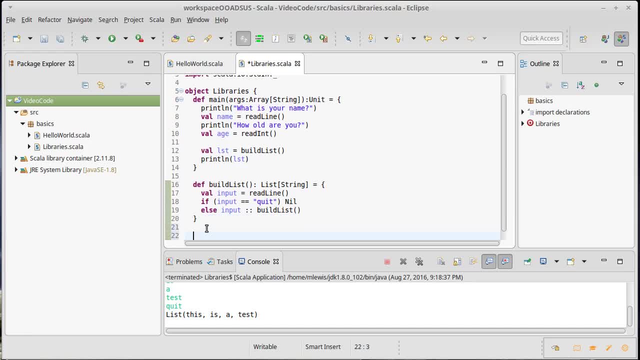 What about going through and, for example, just running through elements? Something that we might want to do might be summing a list of strings. It turns out you can't call sum on the string type. This is something you could do with reduce. 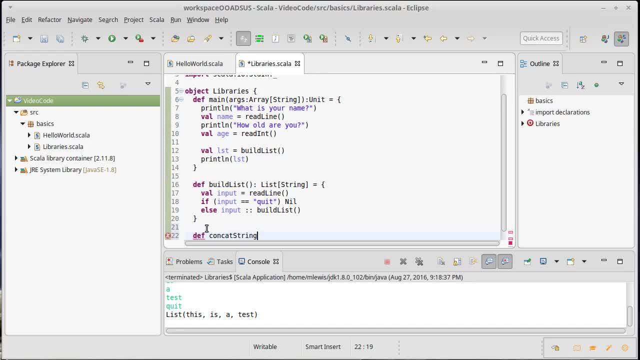 But I want to write a method called concatStrings, which takes a list of string- Actually, I'll probably call it words- And it is going to return to us just a single string. Okay, Well, there are basically two possibilities we want to think of for words. 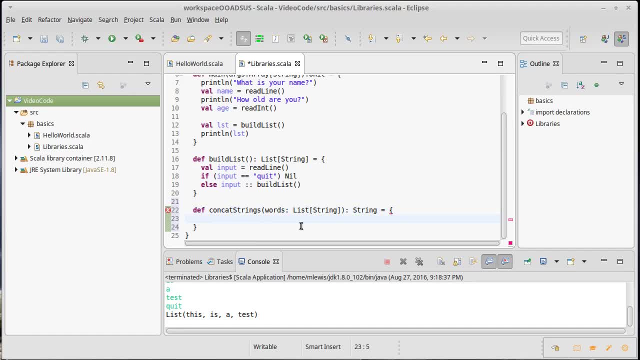 As far as our recursive function goes. One is it's empty, In which case we would return empty string. Otherwise, there is a word there, In which case I should take that word and concatenate it on. Obviously, concatString could also be done with mkString. 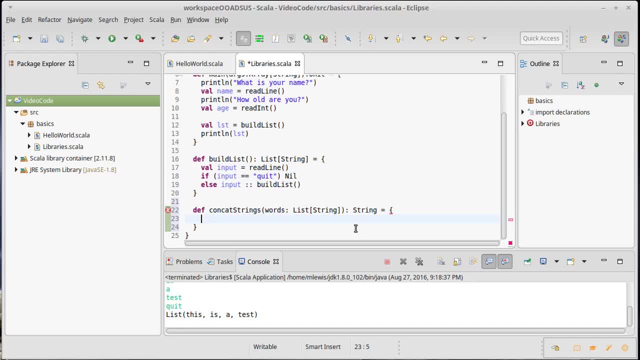 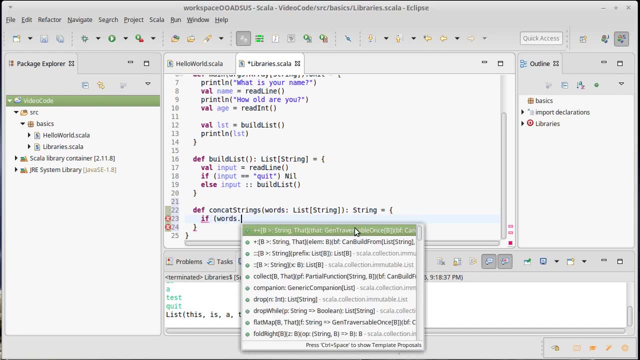 But we want to see how it works recursively. We're going to write this first using an if, So it's. We're going to say if wordsnon, So if there's something there, Actually, no, First let's do words is empty. 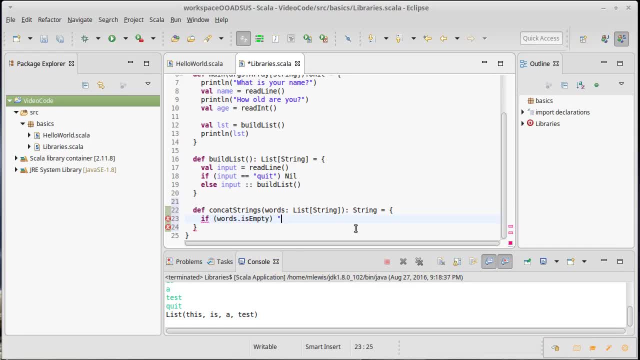 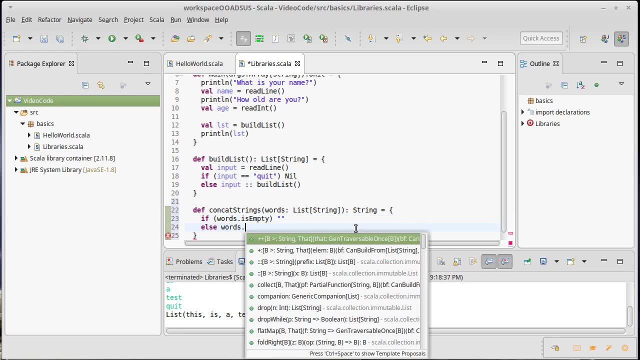 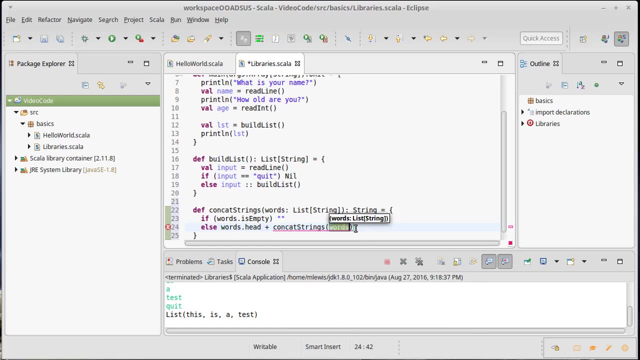 Words is empty. If it's empty, we're going to give back an empty string. Else, we're going to give back the first element Which, remember, we can get by calling head Plus concatStrings. 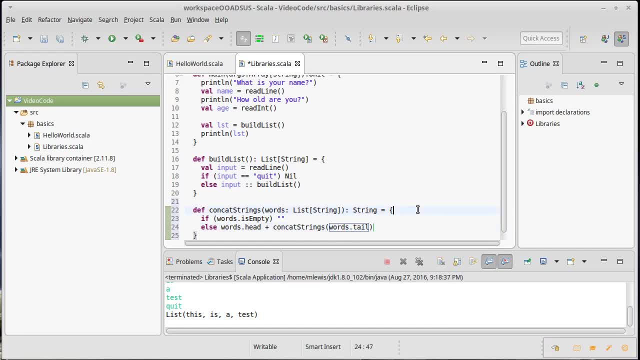 with the rest of the elements, Which we can get by calling tail. So this is perfectly happy code, And we could illustrate this by calling printline of concatStrings. We'll print that instead of what we had before. Now, of course, this is just going to take whatever strings we put in. 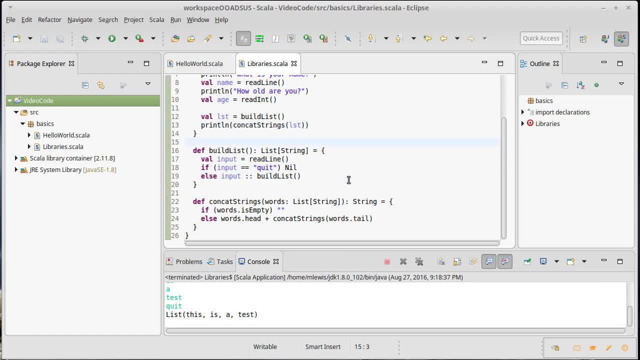 and make a single long string out of them. We run this, Let's input some things there And then let's do again- is a test Quit And it prints out the concatenated. So concatStrings concatenates things together. 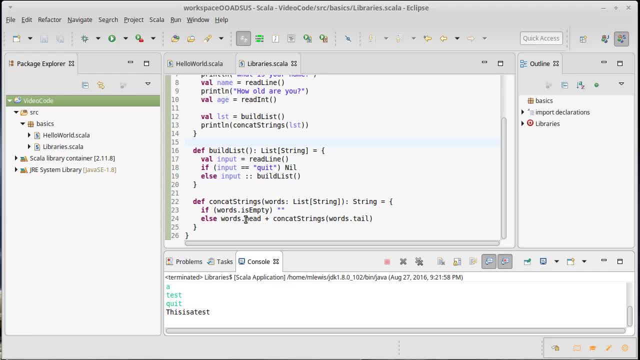 This is using kind of a standard style with an if. to get the first element, we're calling head, to get the other elements we're calling tail. This is all very efficient to do with a list, But there's an alternate way that it's often expressed using patterns. 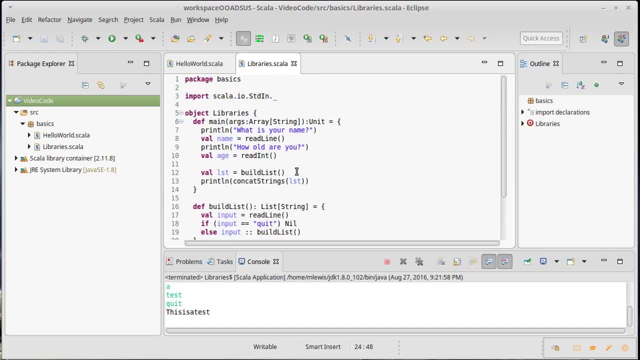 Now, patterns can be used in a number of different places and ways. We saw them- We talked about them a little bit in the match- Turns out you can also put patterns in a vowel declaration. So this is kind of the simplest pattern of just a variable name. 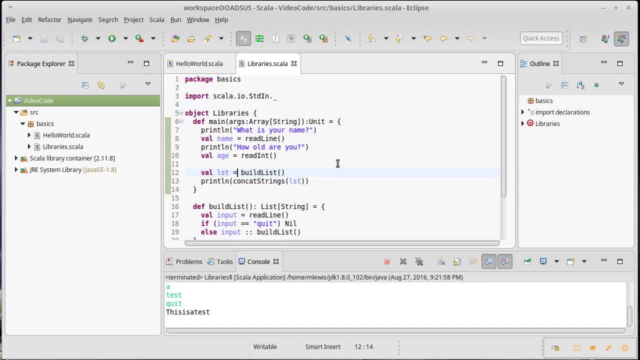 But I could use some other pattern if I wanted. There is also. it turns out that your for loops- the thing before the N arrow on a generator- is a pattern. We'll talk more about that later, because that winds up being very helpful. 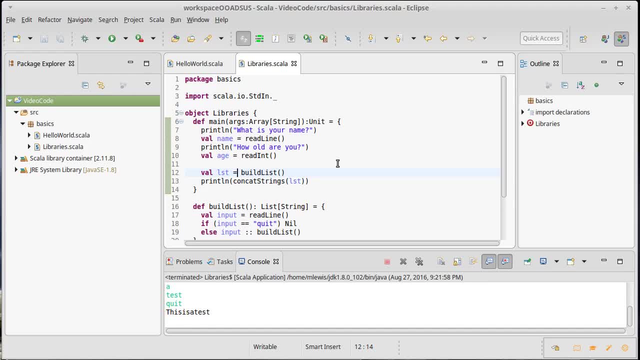 In a number of situations Lists and arrays can be used in patterns. So for example- here's just a simple thing- Array. we'll just say ABC equals one, two, three dot split. 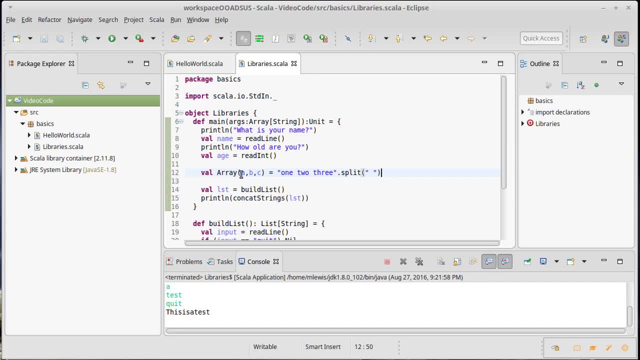 on a space. Okay, So hopefully you can tell what this should do. It's going to take one, two, three. it's going to split them on spaces, which means we're going to get an array with three elements. 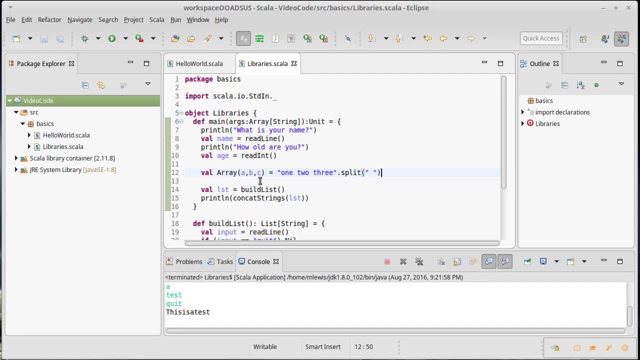 and it's actually going to store those in the variables A, B and C. Now, if this string didn't have three separate values that were separated by spaces, if the result was not an array of link three, 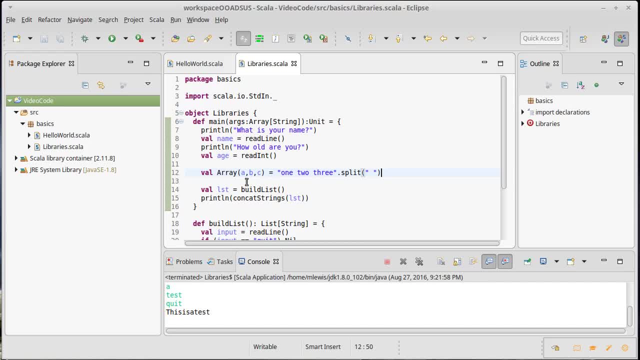 this would crash And that would be. that would be a problem. So you don't. unless you really know what's going to come out from this, you often don't want to do pattern matching quite of this form. 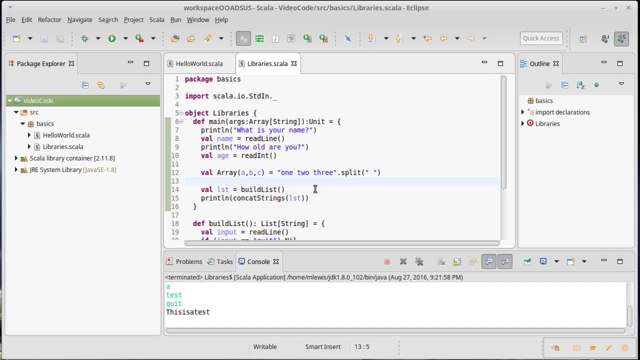 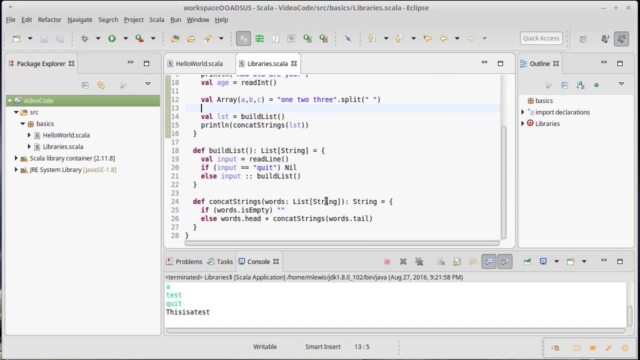 You can do the same thing with lists. If we had a function that produced a list, we could say list and then give it arguments. But that's still not all that general. Turns out you can also do pattern matching using what looks like. 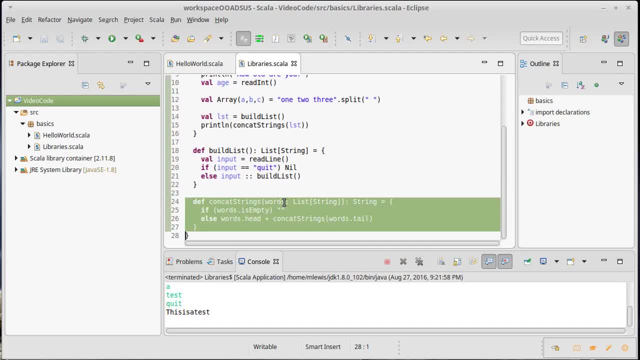 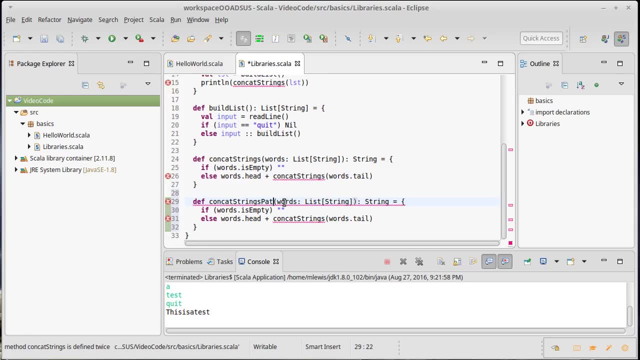 the cons operator. And so we're going to write a second version of concat strings And we're going to call it concat strings- pat Or pattern, And we're going to use a match statement here. We're going to match. 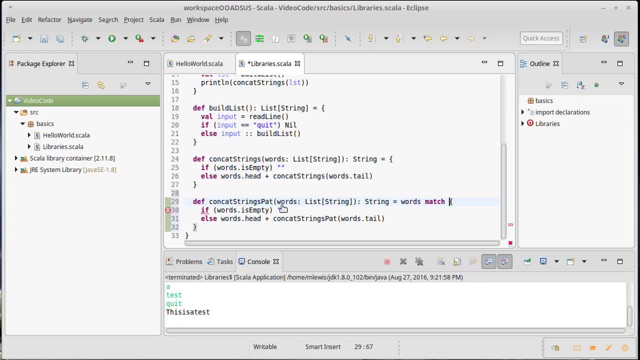 on words, Because the entire body is going to be this one match. I'm just going to put it here after the equal sign and not put an extra set of curly braces. So instead of having an if and an else here, 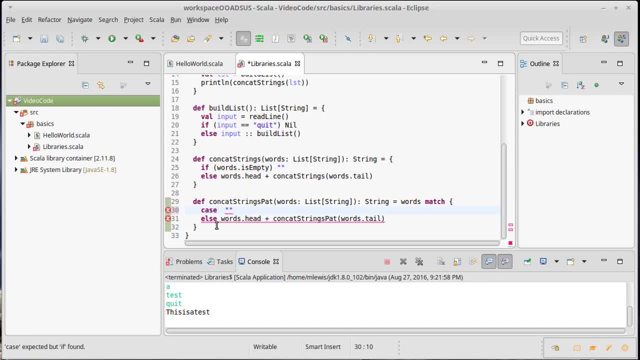 I need cases. So one case is: well, it's empty. As we saw, we can call the empty list by its name, nil. So that's our base case here. The other case can be expressed as a pattern. 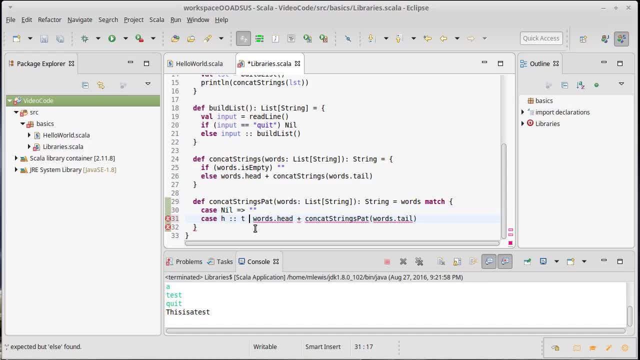 that involves a cons, And we are going to write that as h cons, t- H for head, T for tail, And then, instead of saying wordshead, I say h, And instead of saying wordstail, I say t. 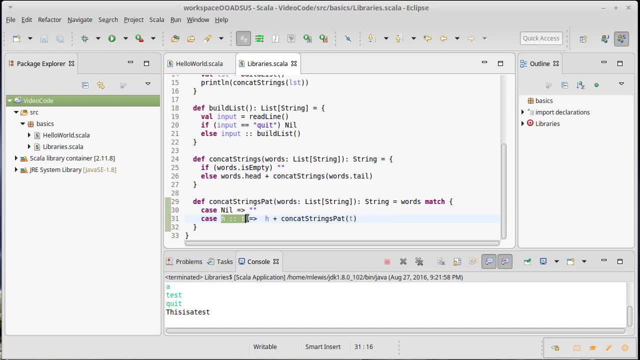 So you can build up these patterns of lists, And I'm not just limited to two, I could have three or four or five. The last thing will always be the tail, for whatever part of the list is left. 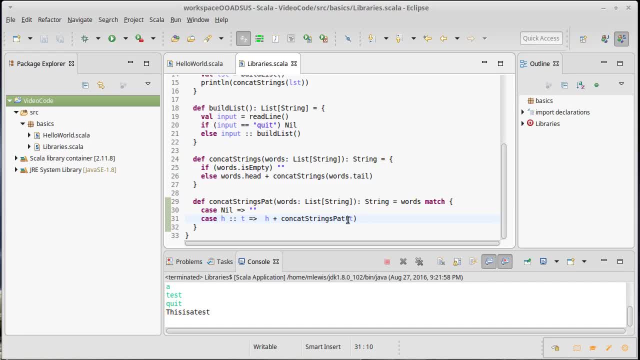 Everything before that will be individual elements, And so you can recurse on the tail And these types of recursive functions. This does exactly the same thing as the concat strings. It's often more common to see, instead of doing ifs. 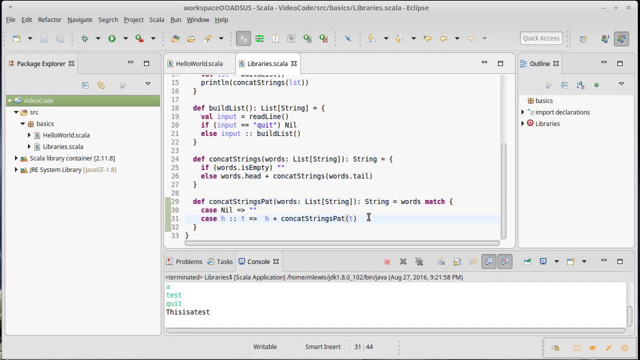 to use pattern matching for pulling apart the strings. So we've talked about lists, We've talked about how lists are used in recursive functions. We've written three different recursive functions that play with lists And we talked about how you can use patterns.